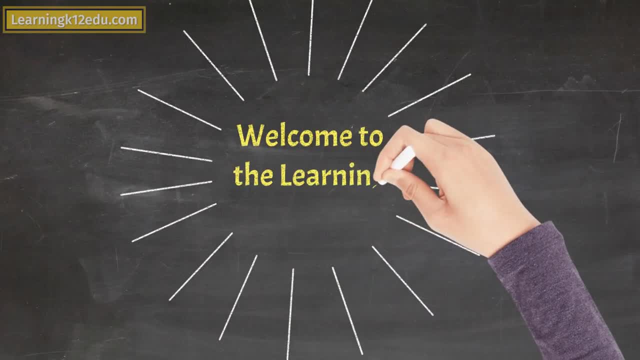 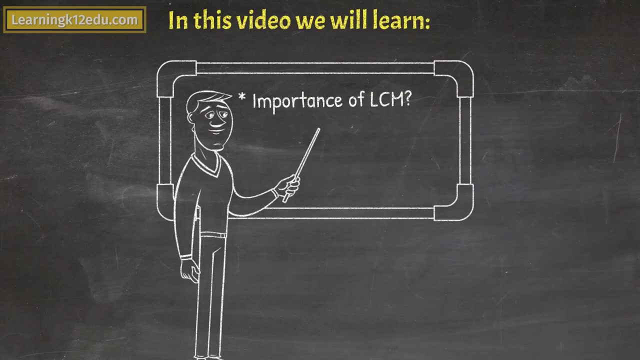 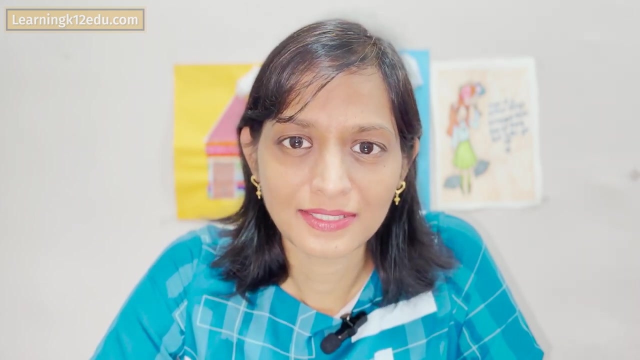 Hello everyone and welcome back to the Learning K-12 channel. Today we will learn about the importance of LCM and real life applications of LCM. I know certain topics in maths are very boring and when I was a child, LCM was top in the list of my boring topics. But now 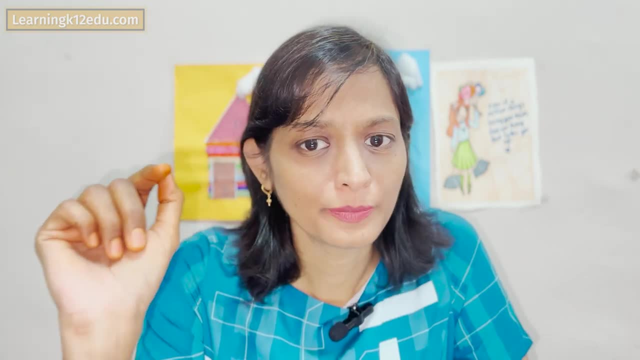 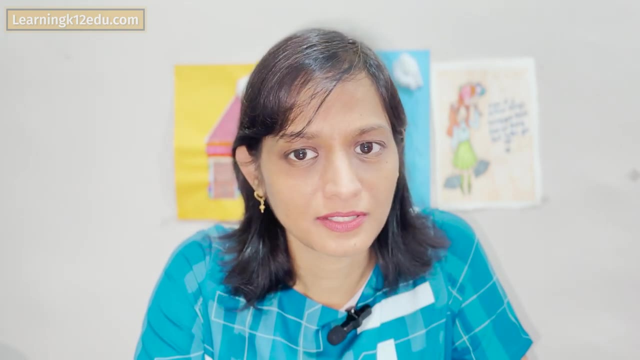 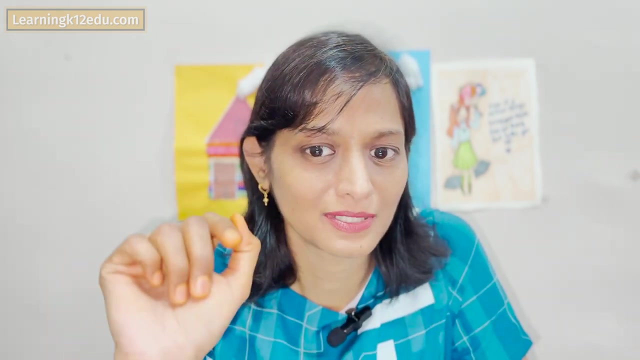 when I think I feel if somebody would have told me the importance of LCM and explained me really well, then probably it would not have appeared in my boring topics list at all. So today I will try to remove this boring topic from your boring topics list. We certainly use LCM in everyday. 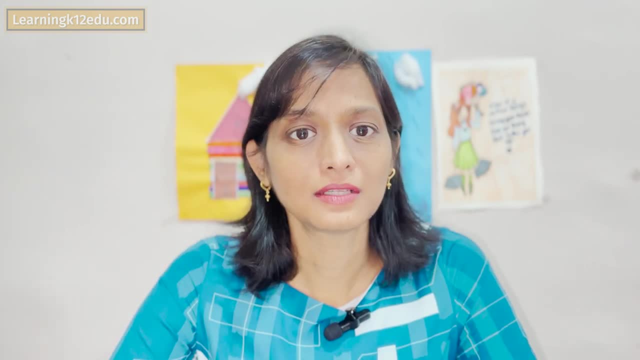 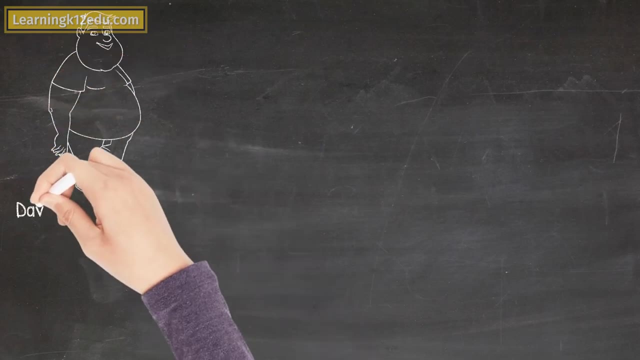 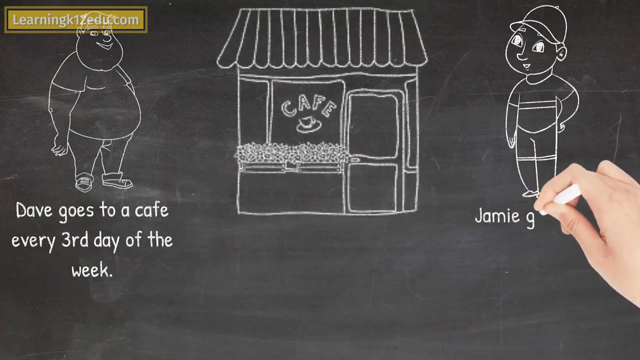 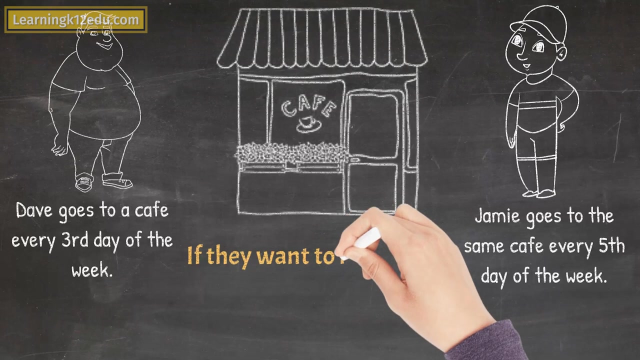 life and we don't even realize it. Let us understand the importance of LCM by analyzing a few situations. Let's take a situation where Dave goes to a cafe every third day of the week but his friend Jamie goes to the same cafe only on the 5th day of the week If they want to meet. 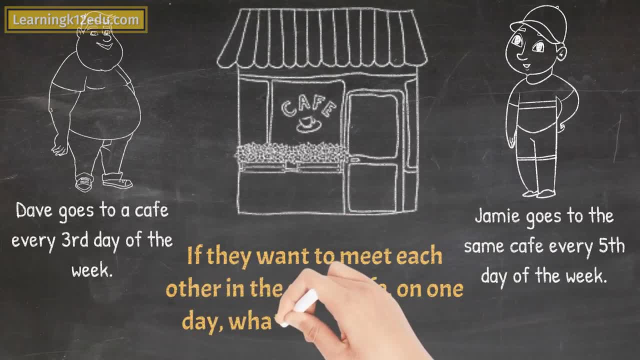 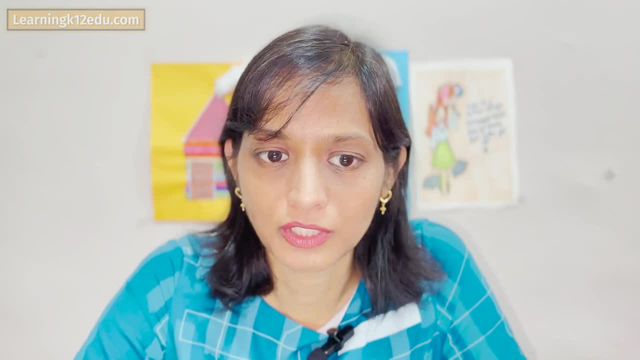 each other in the same cafe on one day, then what day it should be. So how do we find a day that would be common for both of them to meet together? In this case, we need to find the LCM. that would be the smallest thing we have available in our minds. 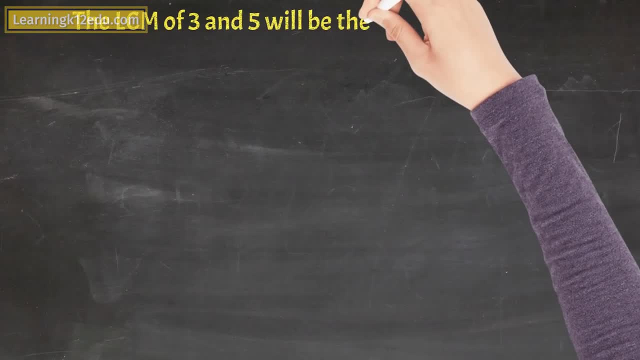 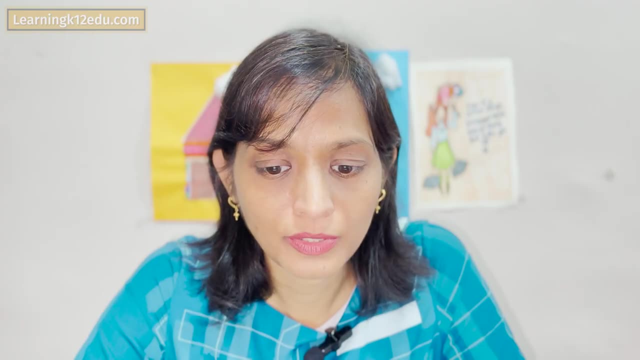 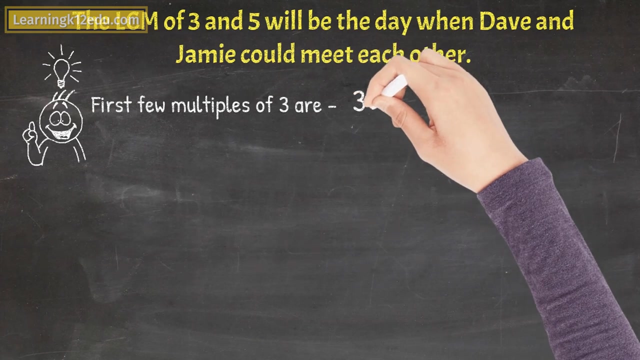 LCM of 3 and 5.. That means the LCM of 3 and 5 will tell us after how many days Dave and Jimmy would be able to meet in the same cafe. So here are the multiples of 3.. 3,, 6,, 9,, 15,, 18,, 21 and so on. 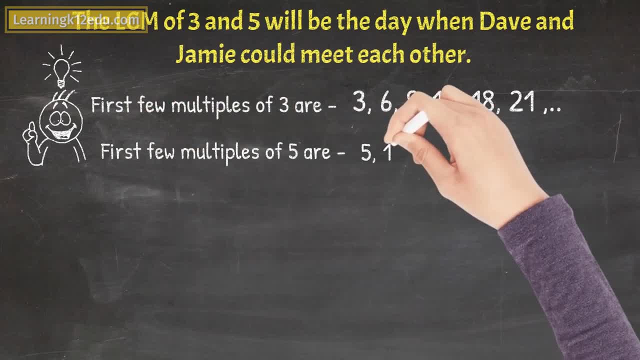 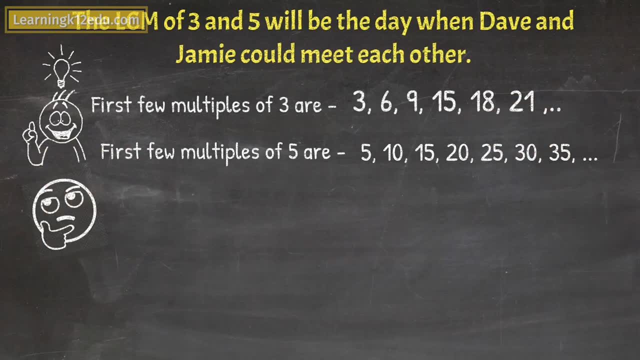 And the multiples of 5 are 5,, 10,, 15,, 20,, 25,, 30,, 35 and so on. As we can see, 15 is the least common multiple among the numbers 3 and 5.. 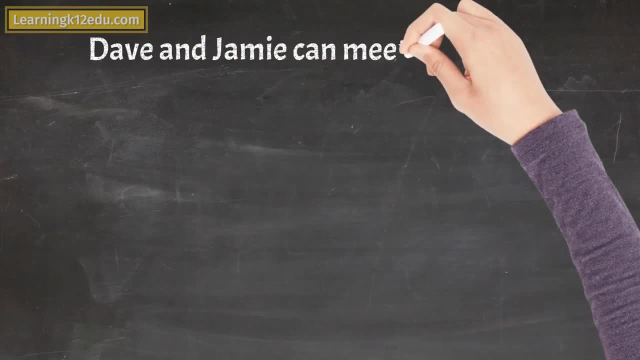 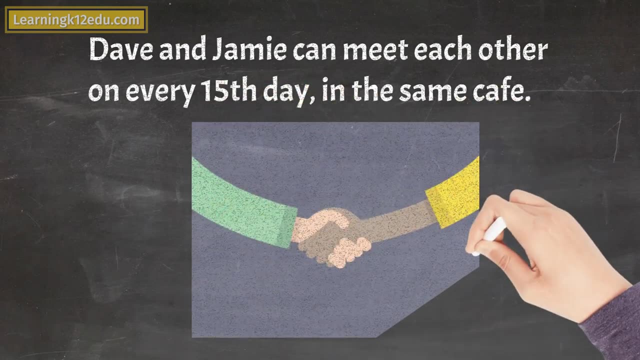 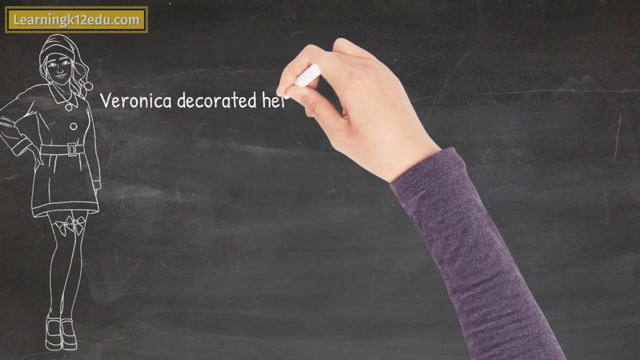 Now we can say: even if Dave goes to cafe every third day and Jimmy goes on every fifth day, they can meet each other on the 15th day. Now lets take another example. Veronica is celebrating Christmas, and for that she has decorated her house with a strip of 900 colorful bulbs. 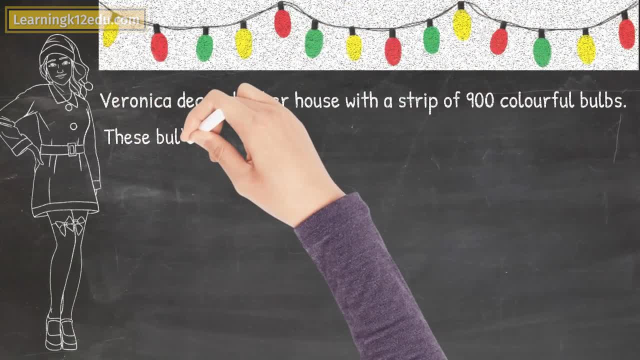 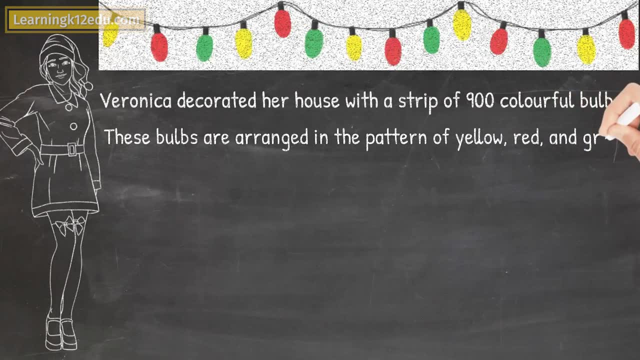 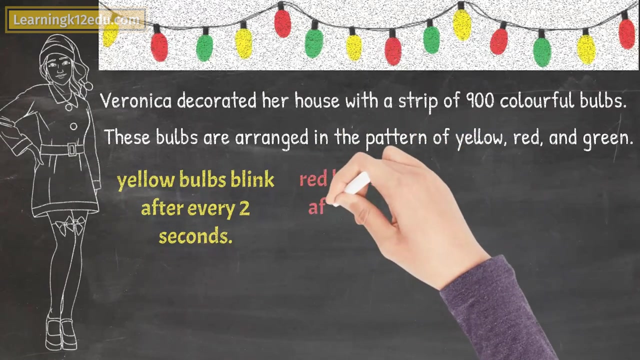 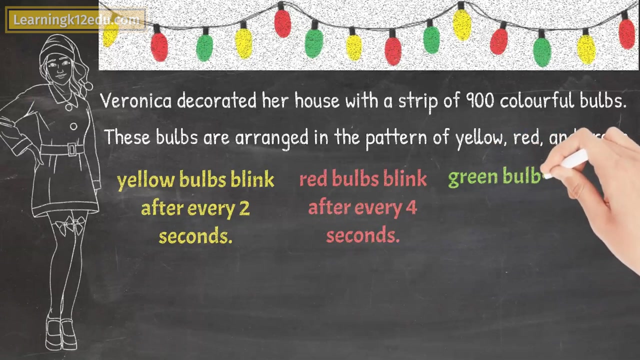 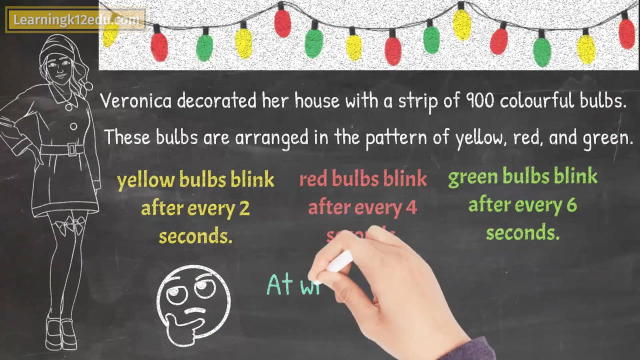 These bulbs are arranged in a pattern of yellow, red and green. All the yellow bulbs blink blink after every 2 seconds, All the red bulbs blink after every 4th second And all the green ones blink after every 6 seconds. At what second all the bulbs will blink together? 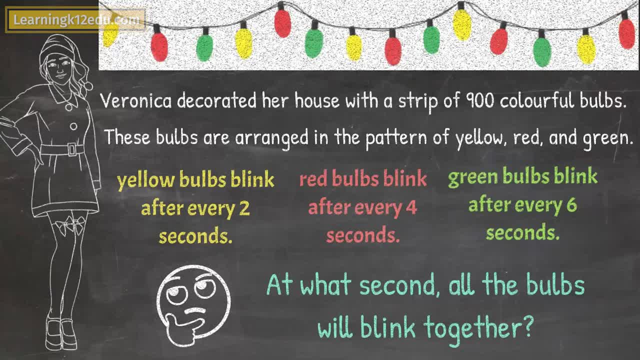 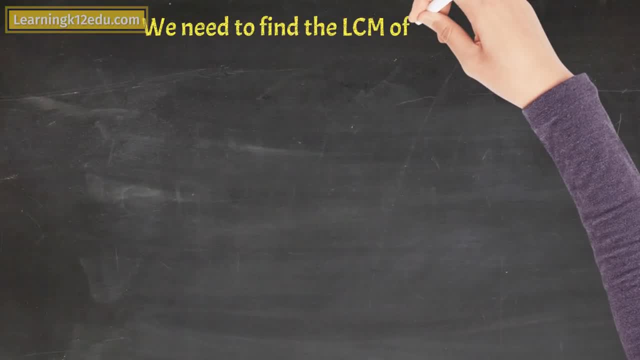 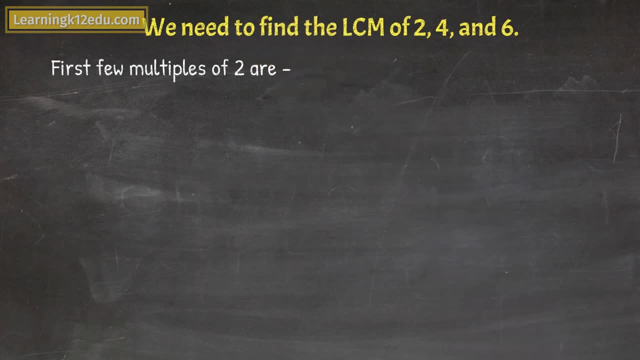 So how do we find a common number at which all the bulbs will blink together? We need to find the first or least common multiple of the numbers 2,, 4 and 6.. Let's see: Multiples of 2 are 2, 4,. 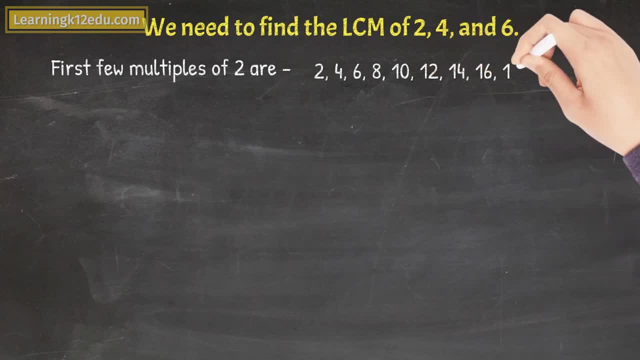 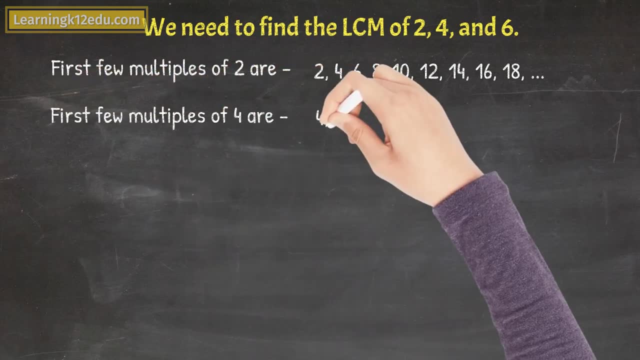 6,, 8,, 10,, 12,, 14,, 16,, 18, and so on. Multiples of 4 are 4,, 8,, 12,, 16,, 20,, 24,, 28,. 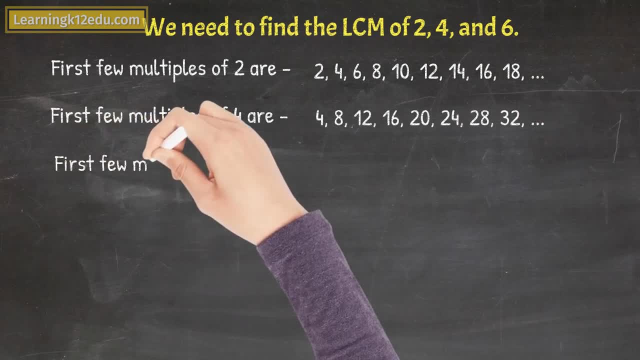 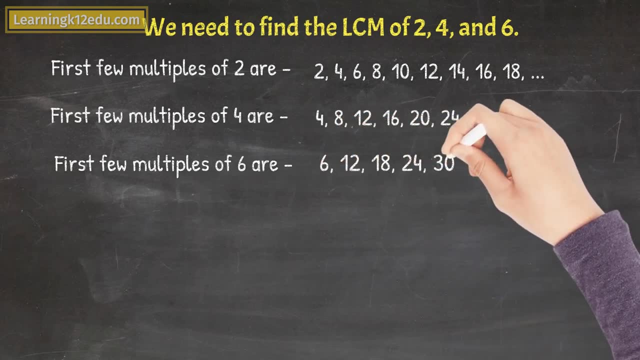 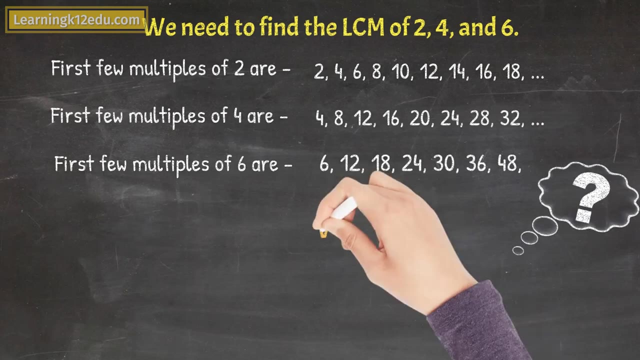 32, and so on. Multiples of 6 are 6,, 12,, 18,, 24,, 30,, 36,, 42,, 48, and so on. Now, as we can see, the LCM of the 3 given numbers is 12.. 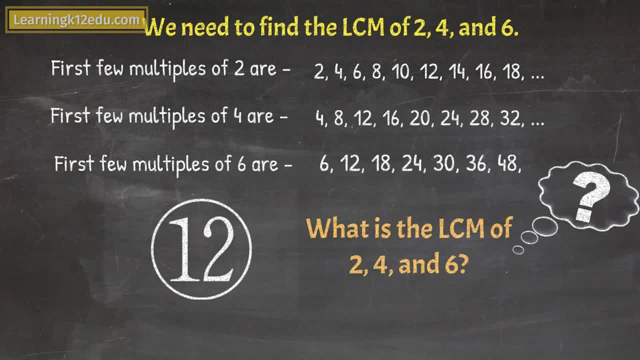 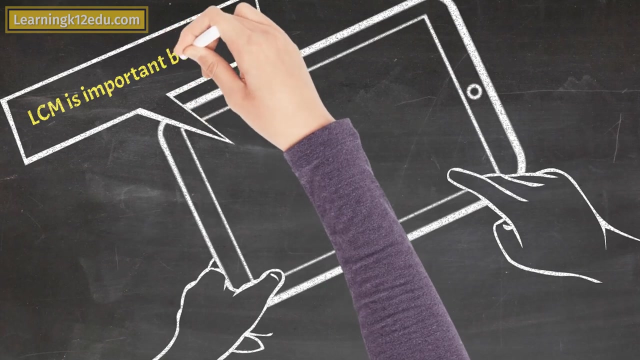 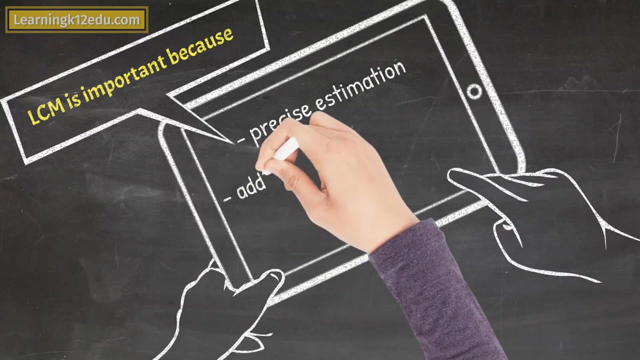 That means at 12th second all the bulbs will blink together. So now we know that LCM makes our life easy and fun, because when we know them we can predict things like magic.